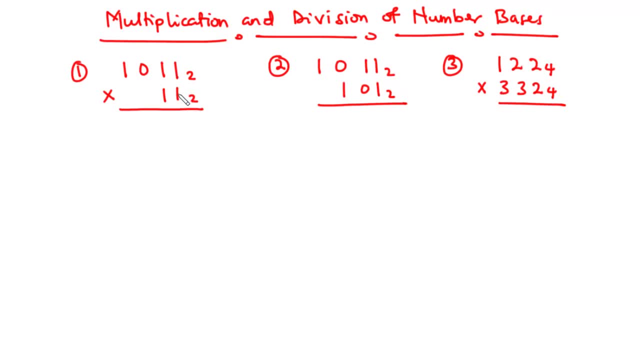 Now let's multiply: 1 times 1 is 1.. 1 times 1 is 1.. 1 times 0 is 0.. And then 1 times 1 is 1.. Now let's move on to the second value: 1 times 1 is 1.. 1 times 1 is 1.. 1 times 0 is 0.. And then 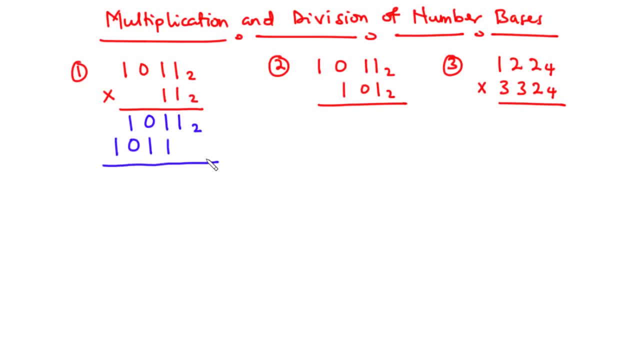 1 times 1 is 1.. Now let's add these two values. We are going to do that in base 2.. 1 plus 0 is 1.. 1 plus 1 is 2.. Now, because we are working in base 2, we can't write 2 here. So we divide 2 by the base And 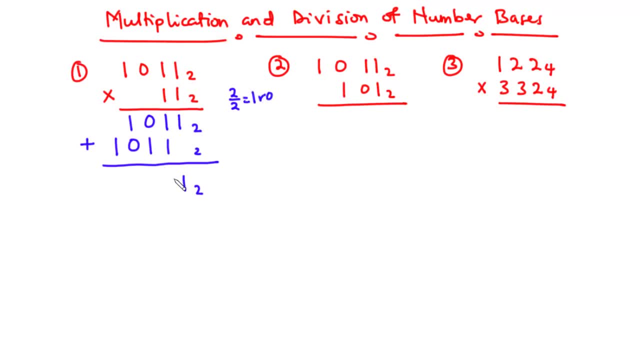 then we have 1 remainder 0. So we are going to write the remainder here And then we carry on. the 1. 1 plus 0 is 1.. 1 plus 1 is 2.. So 2 divided by 2 is 1, remainder 0. So we have. 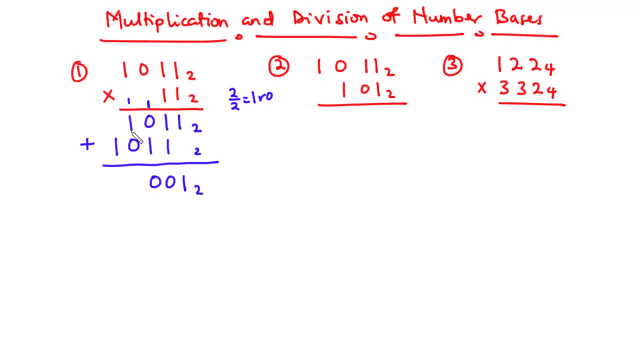 the remainder, and then we carry on the 1.. 1 plus 1 is 2.. Also, we have 0.. And then we carry on the 1.. 1 plus 1 is 2.. So we have 0. And then we carry on the 1.. Therefore, this is going to be. 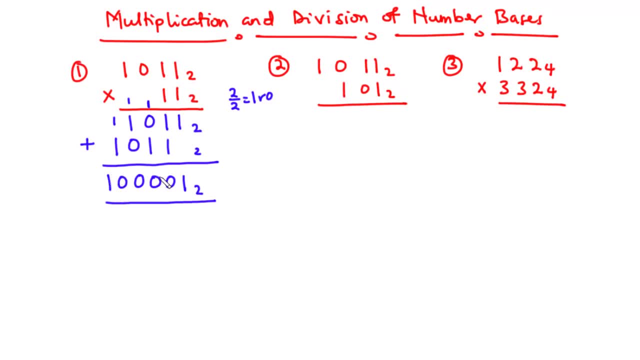 our final answer. Now let's move on to the second example. So for the second example, 1 times 1 is 1.. 1 times 1 is 1.. 1 times 0 is 0.. 1 times 1 is 0.. 1 times 1 is 1.. 1 times 1 is 1.. 1 times 0 is 0.. 1 times. 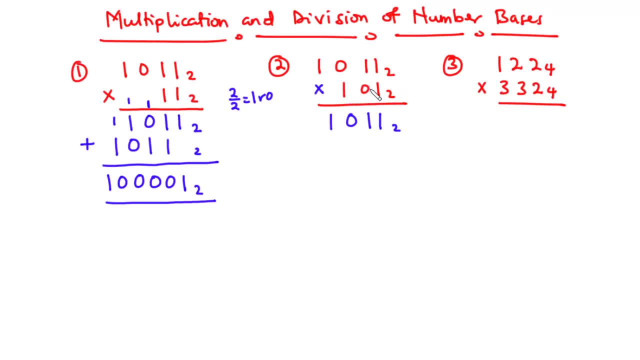 times 1 is 1.. Now to the next value: 0 times 1 is 0,. 0 times 1 is 0, 0 times 0, we have 0, and then 0 times 1 is 0.. To the third value: 1 times 1 is 1,. 1 times 1 is 1, 1 times 0. 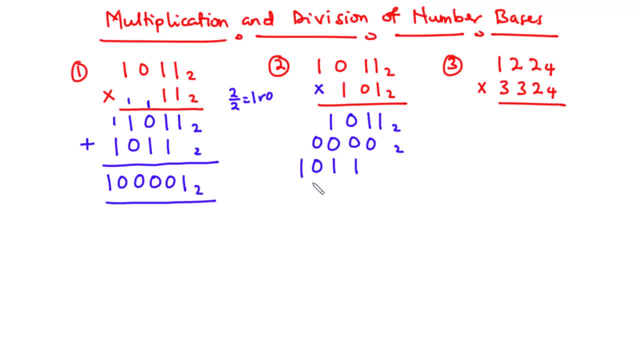 is 0, and then 1 times 1 is 1.. Now we are going to add all these three values in base 2.. So we have: 1 plus 0 plus 0 is 1, 1 plus 0 is 1, 0 plus 0 plus 1 is 1, 1 plus 0 plus. 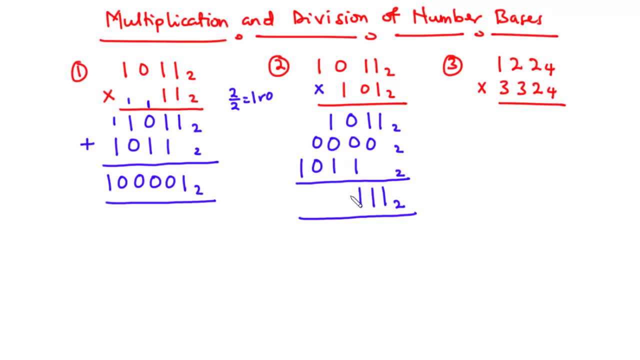 1 is 2.. So 2 divided by 2 is 1, remainder 0. So we have 0, and then we carry on. the 1. 1 plus 0 plus 0 is 1, and then 1 plus 0 is 1.. So this is our final answer. Let's move. 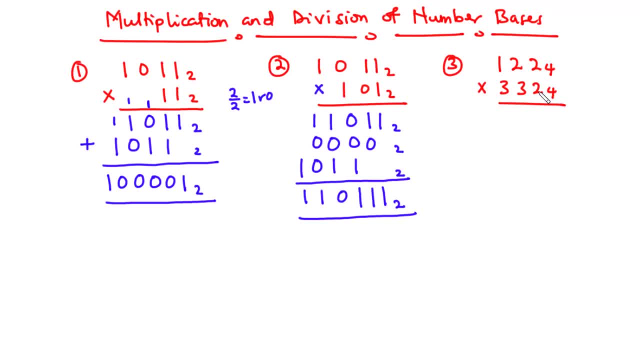 on to the third example. We are going to work in base 4.. 2 times 2 is 4, 4 divided by 4 is 1 remainder 0. So we have 0 here, and then we carry on 1.. 2 times 2 is 4 plus 1 is 5.. So this becomes 1 remainder 1.. So we have 1, and then we carry. 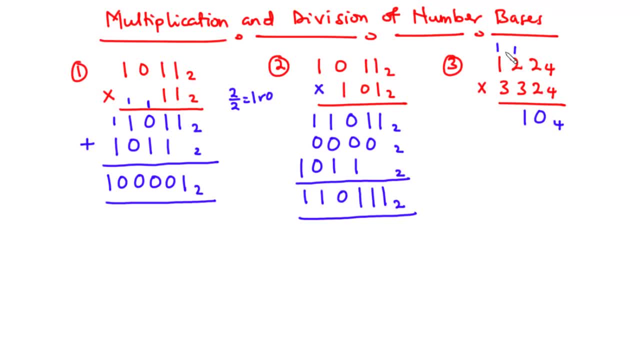 on 1.. 2 times 1 is. 2 plus 1 is 3.. Now let's move on to the second value, which is 3.. 3 times 2 is 6.. 6 divided by 4 is 4.. We are going to work in base 3.. Now we are going. 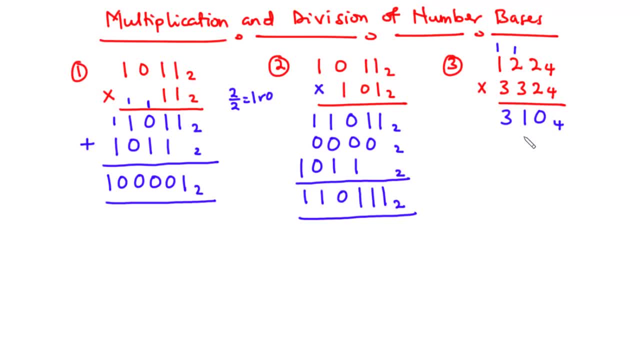 to work in base 5.. Now let's move on to the second value, which is 3.. 3 times 2 is 6.. 6 divided by 4 is 1, remainder 2.. So we have 2 here, and then we carry on: 1.. 3 times 2 is. 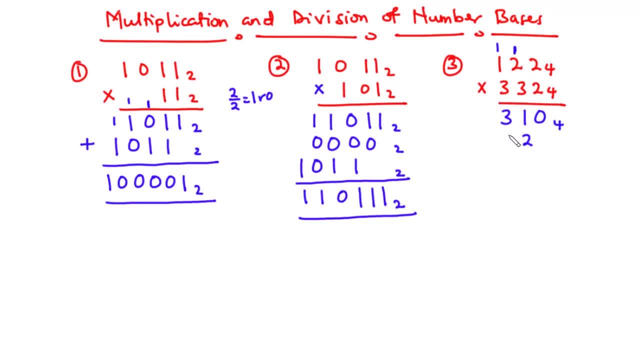 6 plus 1, 7.. So that's going to be 1 remainder 3.. So we have 3, and then we carry on 1.. 3 times 1 is 3 plus 1 is 4.. 4 divided by 4 is 1 remainder 0. So we have 0, and then we carry. 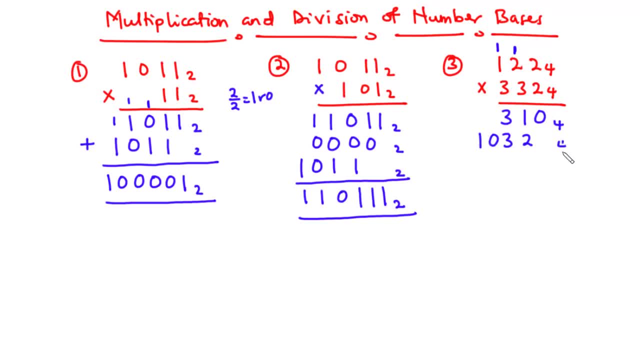 on the 1.. So we have 1,, 0,, 3,, 2.. Now to the third value: 3 times 2 is 6.. So that becomes 1, remainder 2.. So we have 2.. We carry on: 1.. 3 times 2 is 6 plus 1, 7.. So that becomes. 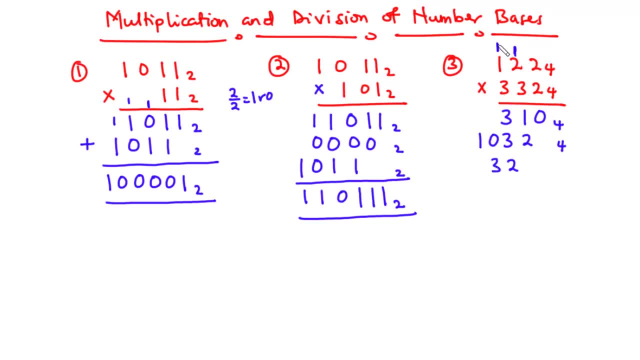 1 remainder 3.. So we have 3.. We carry on 1.. And then 3 times 1 is 3 plus 1 is 4.. So that becomes 0 remainder 1.. So, let's, So, let's, So, let's add the three values: 0 plus 0 plus 0, we have 0,. 1 plus 2 is 3,. 3 plus 3 is 6,. 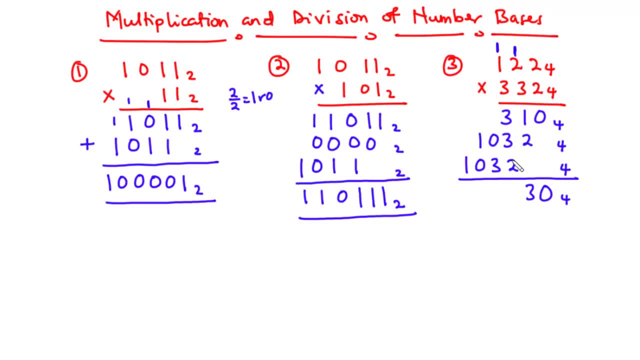 plus 2 is 8, so 8 divided by 4 is 2, remainder 0, so we have 0, and then we carry on 2, 2 plus 0 is 2, plus 3 is 5, so that is 1 remainder 1, so 1, and then we carry on. 1, 1 plus 1 is 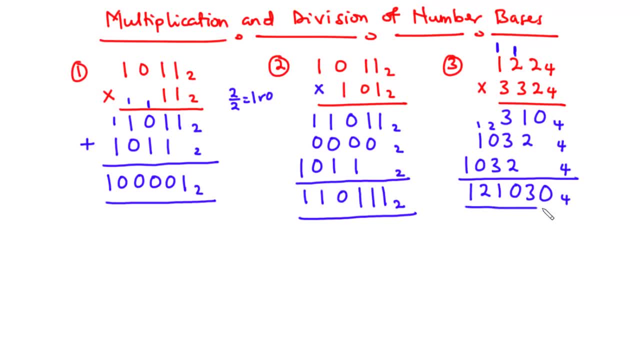 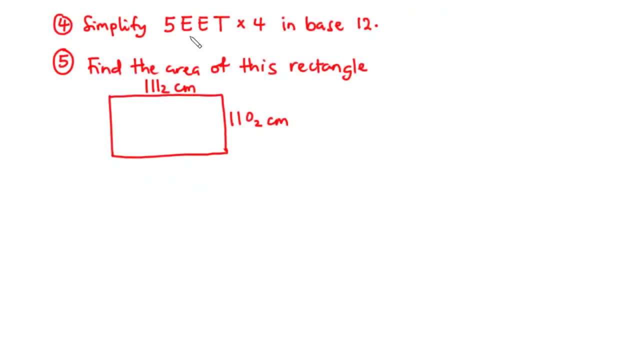 2 and then we have 1 here. So we have our answer to be 121-030, base 4.. Now let's move on as we solve more complex examples. So now to example 4.. Simplify 5EET times 4 in base 12 and then 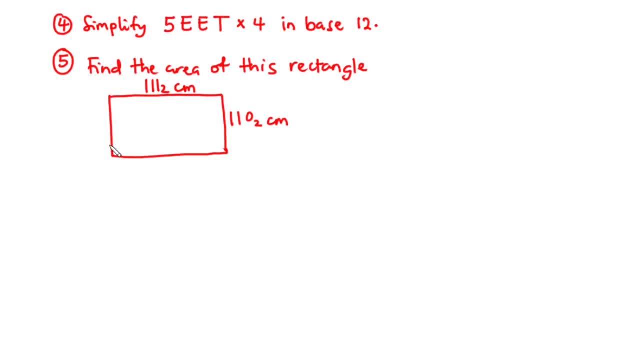 for example, 5, find the area of this rectangle. So we are going to simplify: 1, 5, E, E, T times 4 in base 12.. Now, because we are working in base 12, when you see the letter T, then this represents the value 10.. 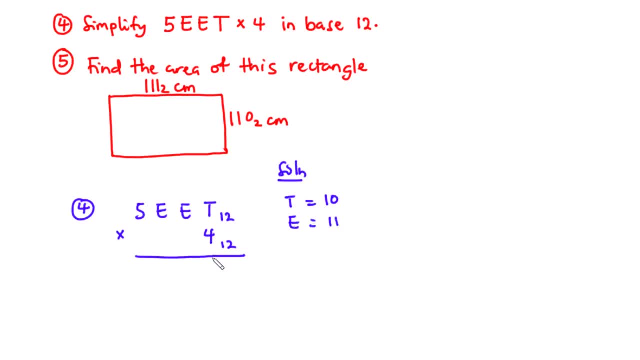 And then when you see E, then that is equal to 11.. So let's take note of that. T times 4 is the same as 10 times 4.. So 10 times 4 is 40.. 40 divided by 12.. 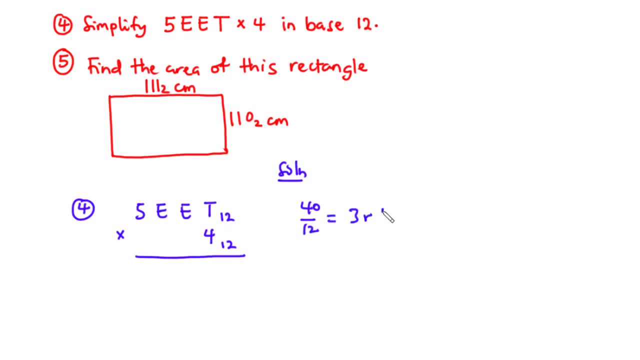 We have 3 remainder, 4.. 12 times 3 is 36.. 40 minus 36 is 4.. So we write the remainder here And then we carry on 3.. E is 11.. So 11 times 4 is 44.. 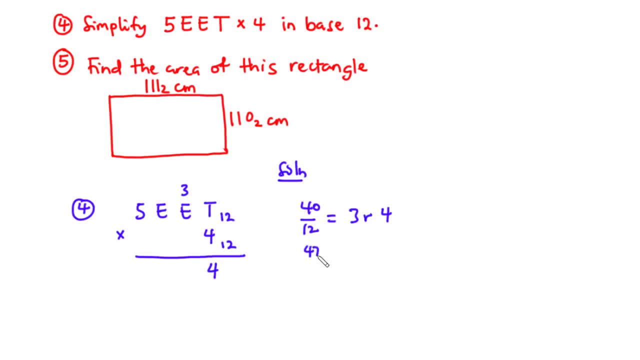 Plus 3 is 47.. 47 divided by 12 is 3, remainder 11.. 12 times 3 is 36.. 47 minus 36 is 11.. So instead of writing 11, we are going to write E. 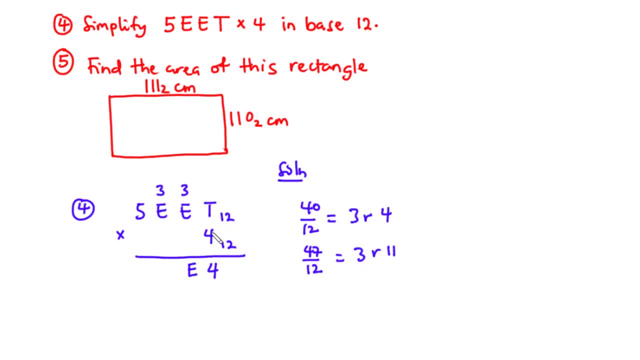 And then we carry on 3.. 4 times 11 is 44.. Plus 3 is 47.. 47 divided by 12 is 3, remainder 11.. So here also We have E, And then we carry on 3.. 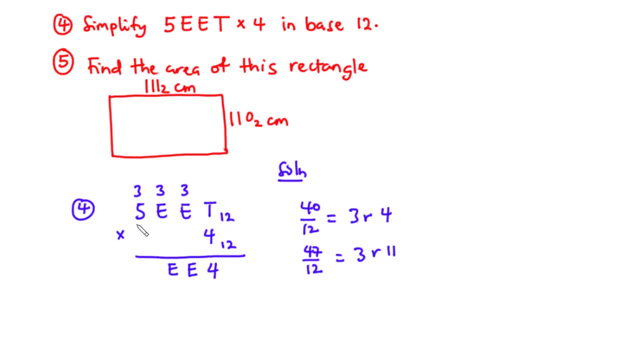 Now, 4 times 5 is 20.. Plus 3 is 23.. 23 divided by 12 is 1, remainder 11.. 12 times 1 is 12.. 23 minus 12 is 11.. So we have 11 here. 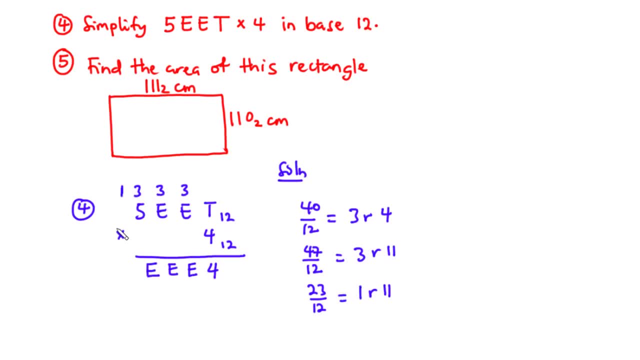 And then we carry on: 1.. So we have 1 here, And this is our final answer. 1, E, E, E, 4, base 12.. Now let's move on to example 5.. So, for example 5, we are going to find the area of this rectangle. 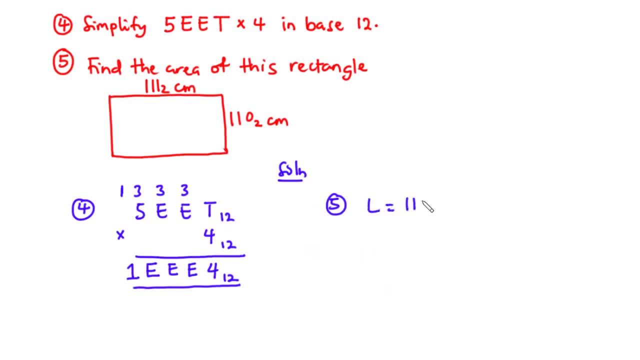 Now we have the length to be 111 in base 2 centimeters, And then we have the breadth to be 110 base 2 centimeters. We know that the area of a rectangle is given by length times the breadth. Therefore, we have 111 base 2 times 110 base 2.. 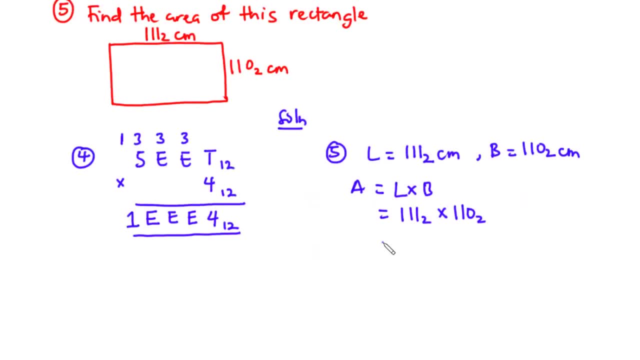 Now let's multiply the two values, So we have 111 base 2 times 110 base: 2.. 0 times 1 is 0.. 0 times 1 is 0.. 0 times 1 is 0.. 1 times 1 is 1.. 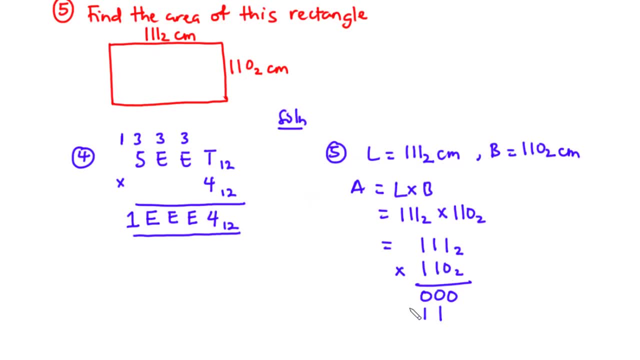 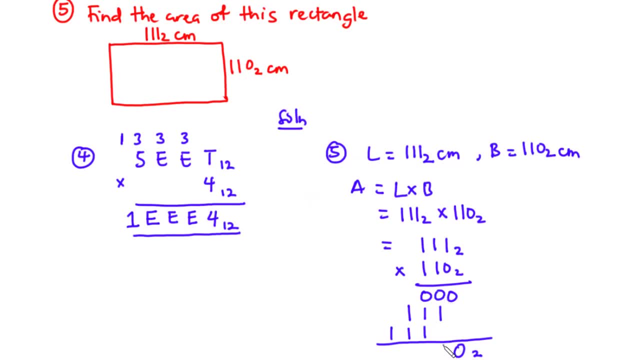 So we have 0.. 0 plus 1 is 1.. 0 plus 1 is 1. Plus 1 is 2.. So we have 0.. 1 plus 1 is 0.. 0 plus 1 is 2.. 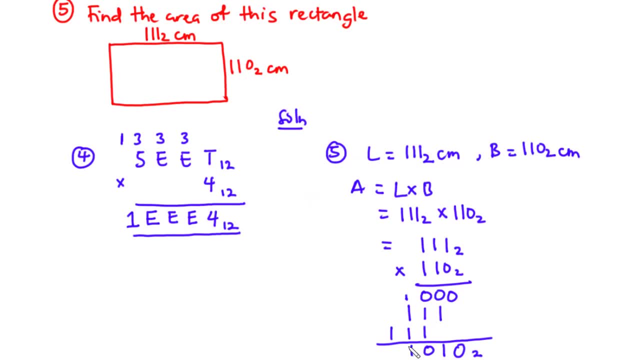 1 plus 1 is 2.. 2 plus 1 is 3.. We have 1, remainder 1.. And then 1 plus 1 is 2.. So we have 0 and then we carry on 1 here. Therefore, the area of this rectangle is 101010 cm in base 2.. 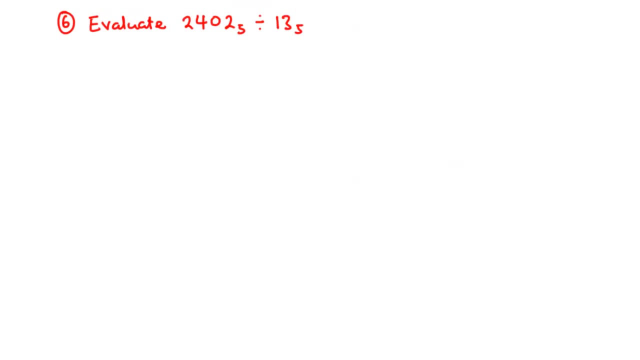 Now to example 6.. We are going to evaluate 2402 base 5 divided by 13 base 5.. So for division, it is very confusing to do that straight away. However, the best thing to do is to convert all these values to base 10 and then we perform the division. After that we convert the result back. 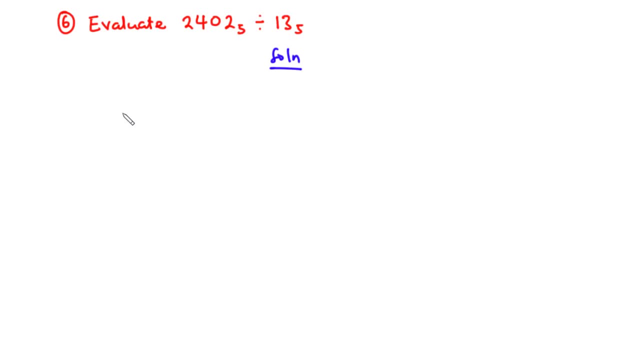 to base 5.. So that is exactly what we are going to do. Now let's see how we do it. Let's convert 2402, base 5, to base 10.. So that's going to be 2 times 5 plus 4 times 5 plus 0 times 5 plus 2 times 5.. 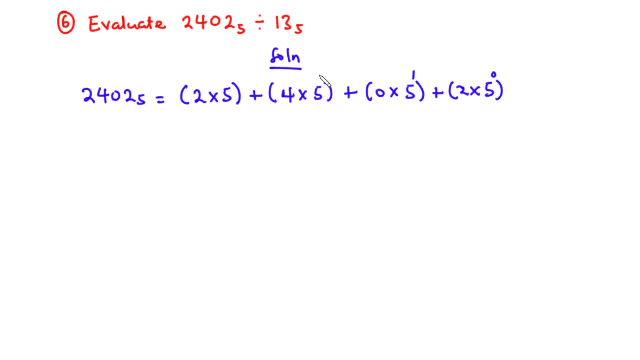 So, starting from the right hand side, we have 0,, 1,, 2 and then 3.. Now let's simplify: 5 exponent 3 is 125.. Times 2,, we have 250.. 5 exponent 2 is 25 times 4 is 100. 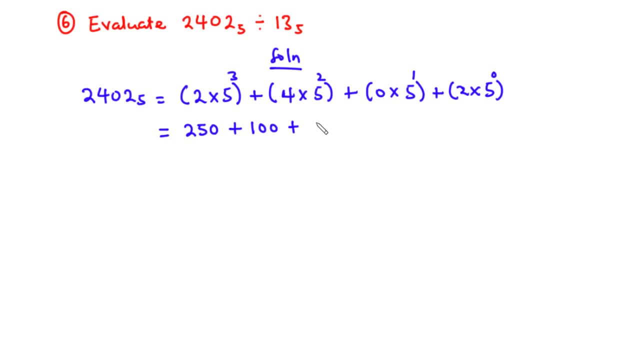 5 exponent 1 is 5 times 0 is 0, 5 exponent 0 is 1 times 2 is 2.. So 250 plus 125.. It's 90+. 300 plus 0 plus 2 is 352, base 10.. 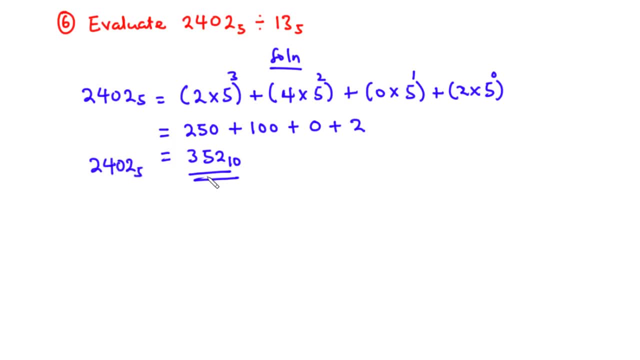 So 2402 base 5 is equal to 352 base 10.. Now let's work on the 13. So 13 base 5 is also equal to 1 times 5 exponent 1 plus 3 times 5 exponent 0.. 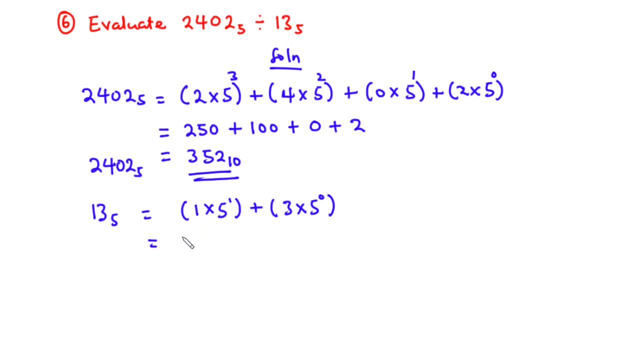 So this also becomes: 5 exponent 1 is 5 times 1 is still 5.. 5 exponent 0 is 1 times 3 is 3.. So we have our final answer to be 8 base 10.. Now let's divide 352 by 8.. 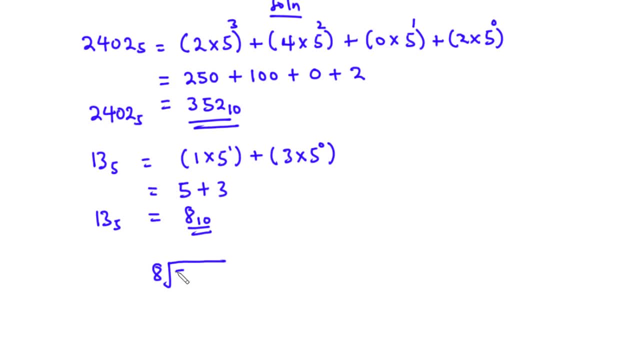 So we have 8 on the outside and then 352 under the square root. Now 8 goes into 35. four times 8 times 4 is 32,. 5 minus 2 is 3,. 3 minus 3 is 0..